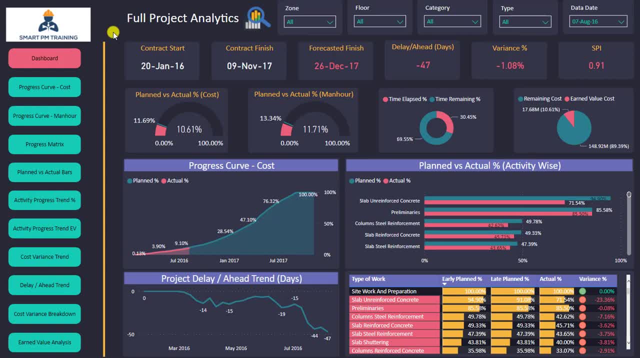 This is my dashboard and I have here my key progress indicators: contract start, contract finish, forecasted finish, the amount of delays, the variance percentage, SPI, planned versus actual, based on cost and based on man hours, The time elapsed and time remaining percentages, the remaining cost and earned value cost. This is an overview of the progress curve based on cost, and I have here as well the planned versus actual percentages and I can scroll down to see all activities in my project. 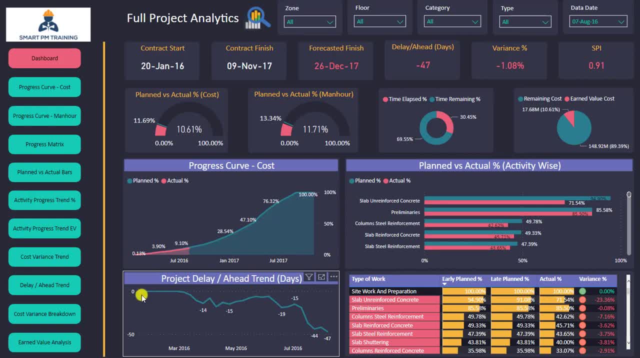 And here I have the trend of project delays. During this period I had no delays in the project. Then the amount of delays remained stable during this period. Then I had more significant delays over time. This is my progress matrix. I have here the list of activities, the planned percentages as per early date and as per late dates as well. 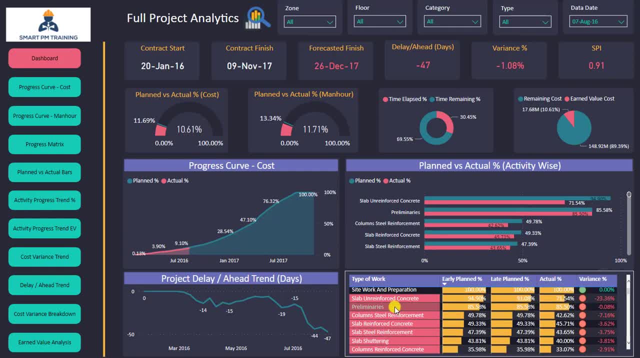 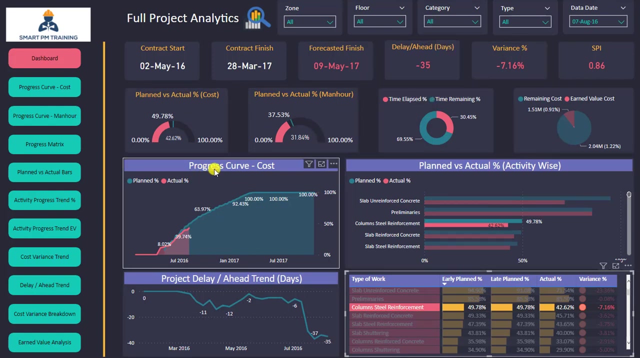 The actual percentage and the variance percentage and I can scroll down to see all activities listed in the project, and the delayed activities are highlighted in red and I have the indicators here as well to tell me whether or not the activity is in delay. Not only that, I can click any activity and the whole dashboard will be interactive with me. So the progress curve right now will respond to my selection and all my indicators here will change to reflect the columns. steel reinforcement only. 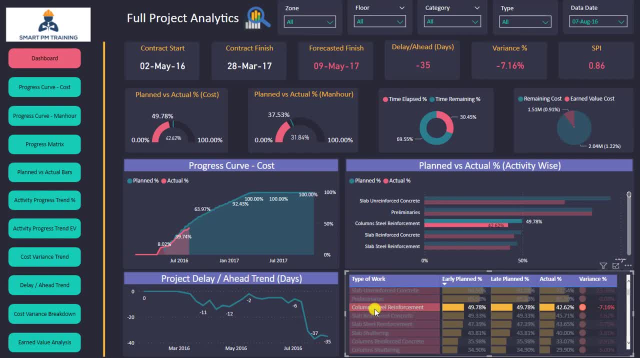 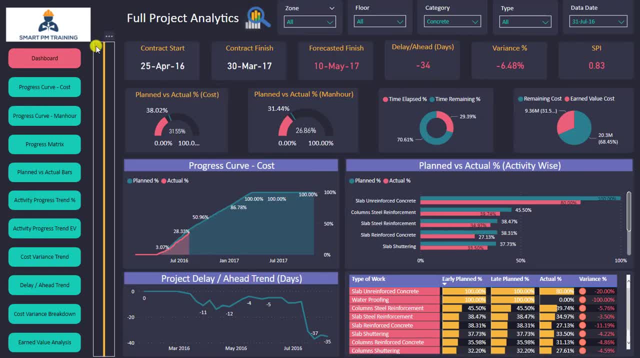 I can see also that the part related to the columns- steel reinforcement, is highlighted in this chart, and it will show me how much the earned value and the remaining cost will be reflected in this chart. The 자기-speculation dashboard is meant to show high level information. 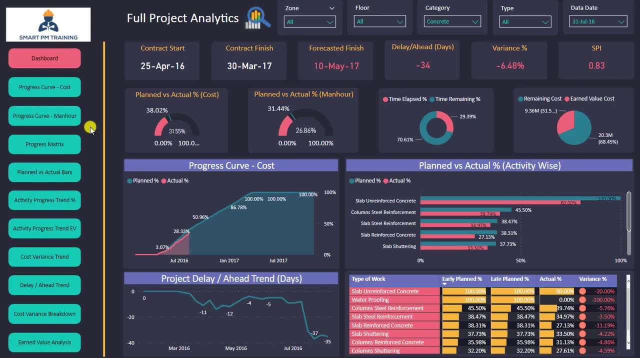 What I'm gong to show you now is how you can carry out more complex and advanced analysis. You can basically do anything you want in project control of your project with one click. You can basically do anything you want in project control of your project with one click. 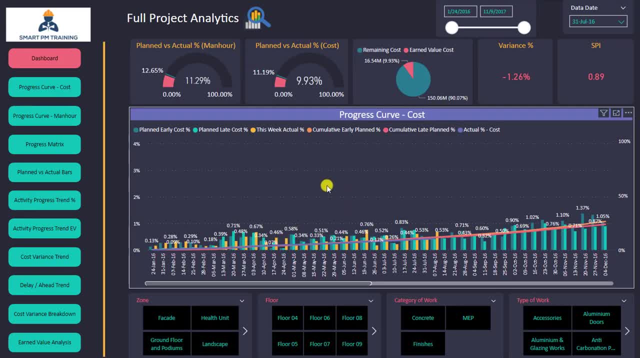 Let's go to the progress curve. Let's go to the progress curve. And this is the detailed progress curve for everything. I can see here the planned percentage on weekly basis, based on the early and delay date, the actual as well. And this is the detailed progress curve for everything. 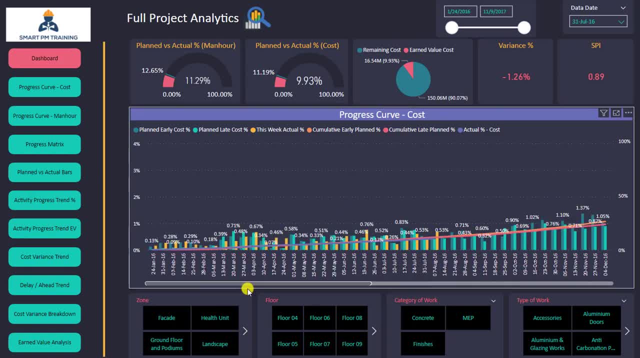 as well as the planned percentage on weekly basis based on the early and delay date, well as the cumulative for planned and actual. but what if i am not interested to see all the information here? i wanna only analyze this part of the chart. i can use the slider here to select. 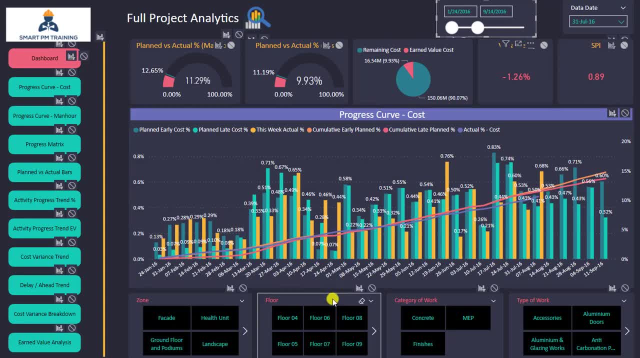 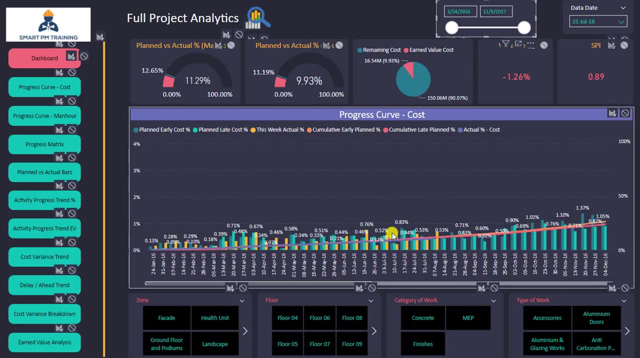 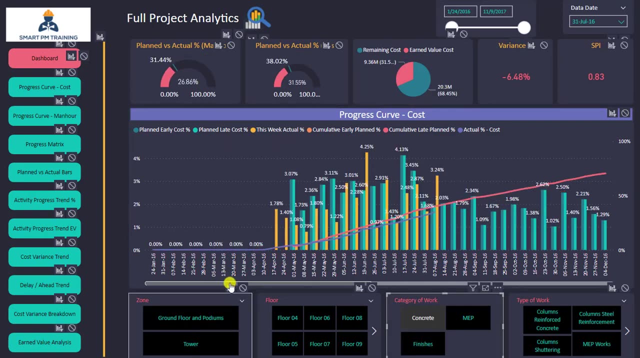 the timeline and i can now have a better understanding and better visualization of the progress during the selected period. only, not only that, i can go to any filter of my choice here. let's go to concrete, for example, and now i have the progress curve for the concrete category. 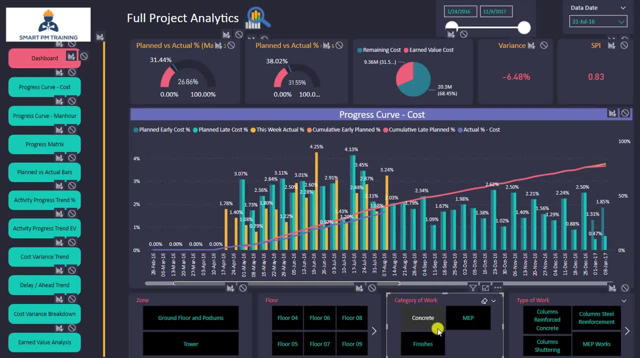 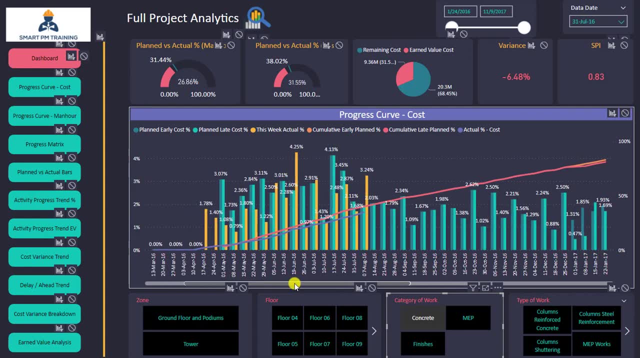 only so. in other words, in this case i will consider the concrete as a separate project with its own contract value and timeline, and the progress curve will be generated for me immediately, with one click only. so now i can see the progress curve for the concrete. these are the 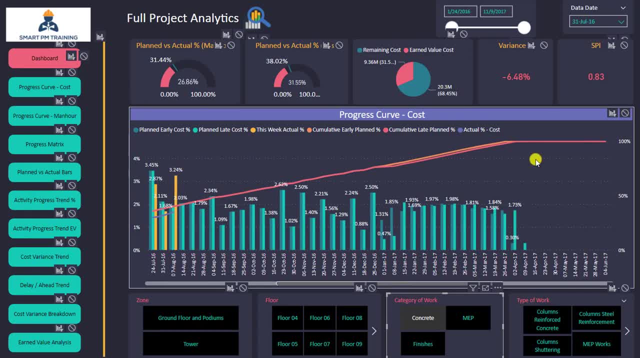 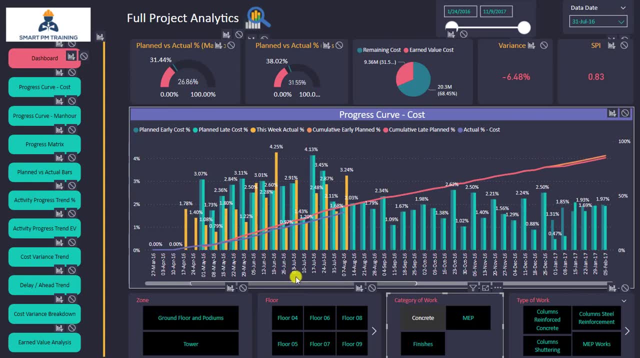 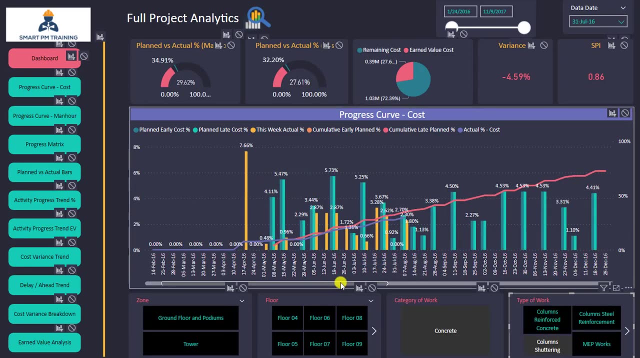 percentages for the concrete work only and also the cumulative for the concrete, the timeline for concrete. so now i have laser focused analysis of concrete activities, i can do whatever i want, column shutterings, for example. i can now have the progress curve for column shuttering only with the 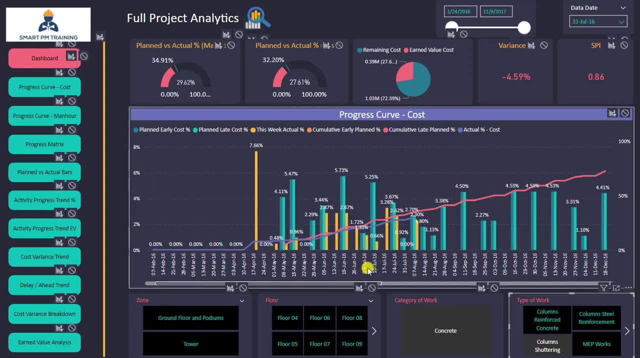 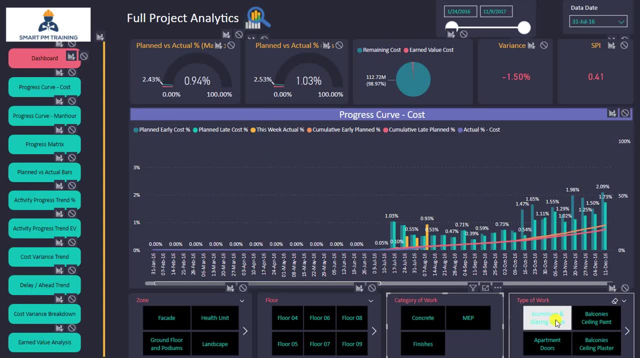 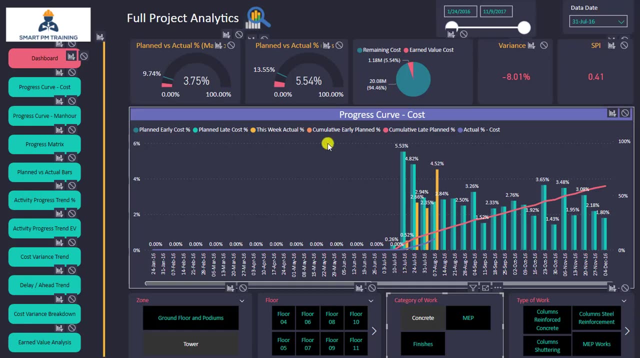 planned versus actual trends. so this is very powerful and it depends on the level of detail you wanna analyze. the s curve will be generated for me: planned versus actual, and if i select the concrete activities, i can also see the progress. indicators are interactive with me, so it's updated based on my selection right now and i can go to column steel reinforcement. 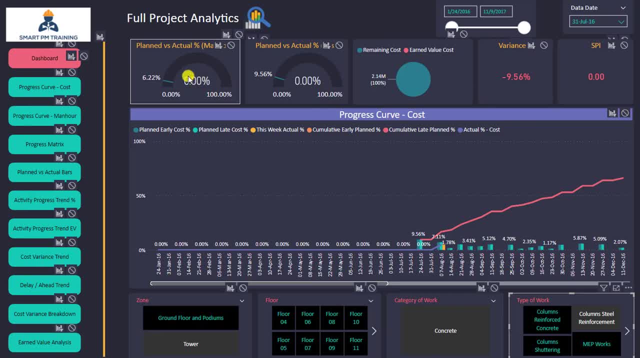 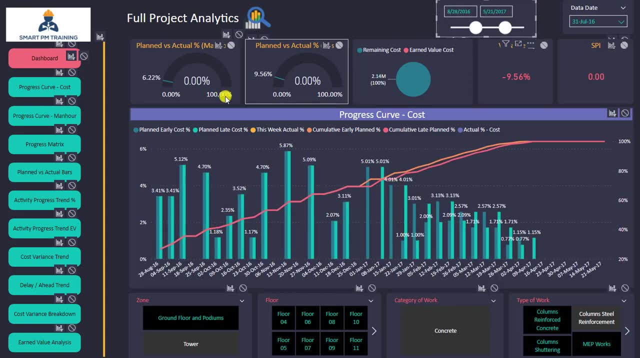 i can see here from the indicators that no actual percentages, but i have some planned percentage. it's obviously in delay. i can also use the slider again anytime i want. so everything is working, is synchronized. i can also do the same level of analysis, but based on man hour. 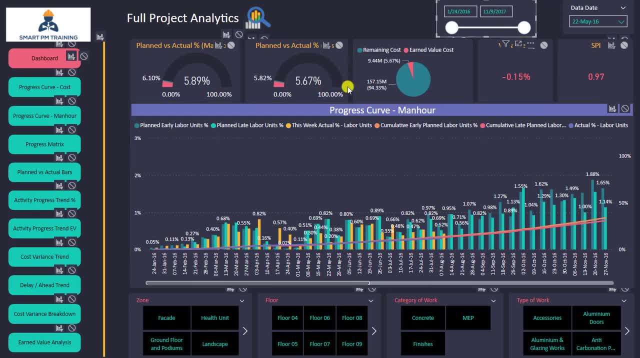 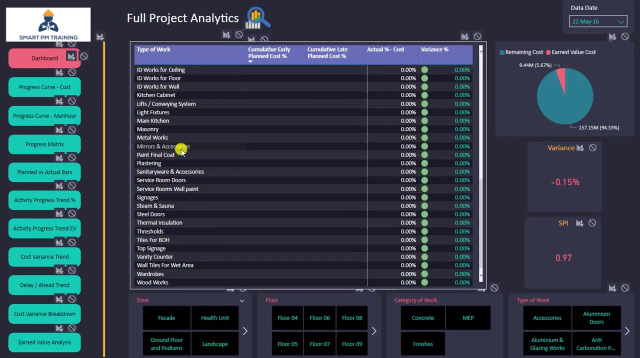 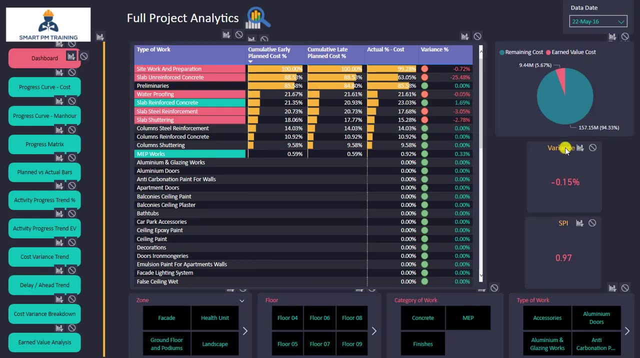 so it's the same layout, but everything here is based on man hour. i can go now to the progress metrics and i will see the list of activities for the whole project. what is the planned versus actual and what is the variance? the same indicators here related to the earned. 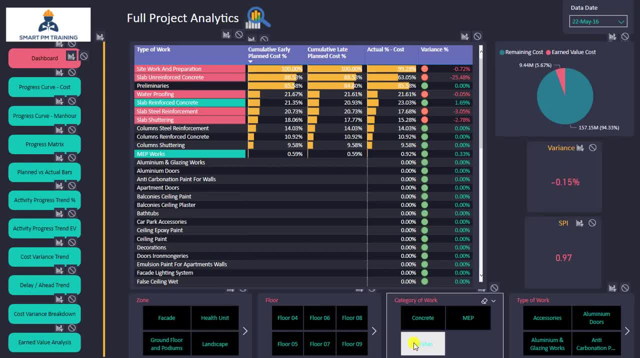 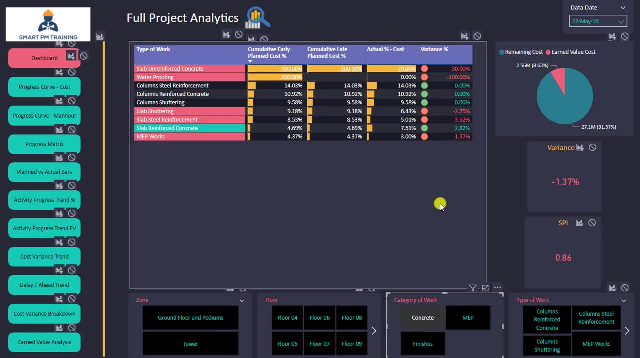 value, variance percentage and spi. i can also choose concrete, for example, and it will filter only concrete activities. so i can have a better analysis of it and i can also go back at any point of time, as we have seen before, to see the status. then all the indicators will reflect. 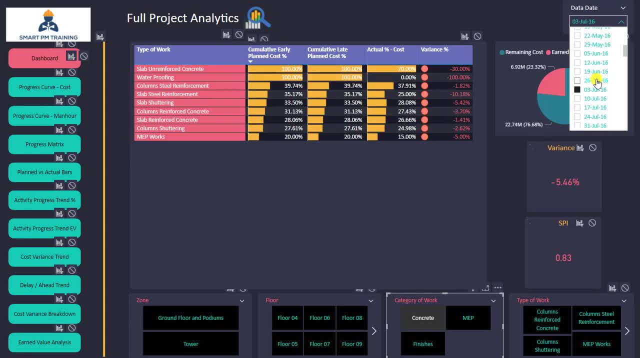 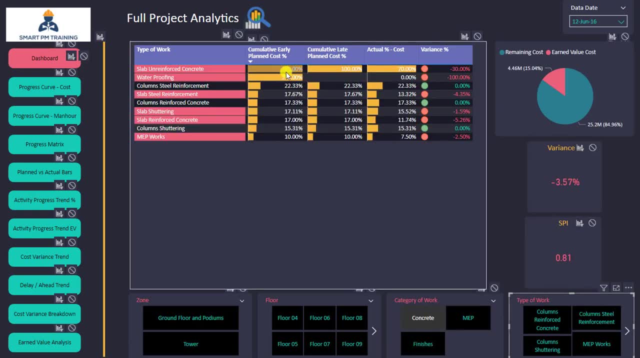 progress status for the selected data date. so anything i choose here, they are all working okay and i can basically choose everything. columnister reinforcement and the orange bars here are generated automatically to indicate the strength of the value. so 100 it's a full bar, followed by 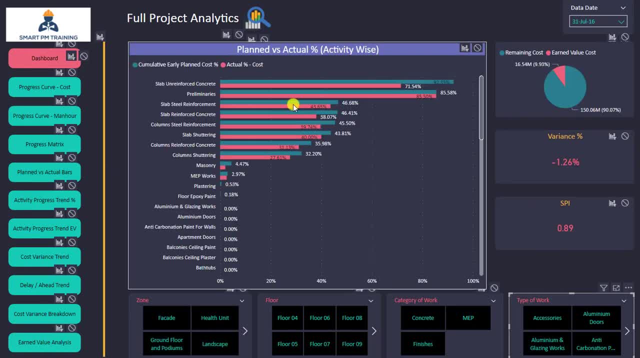 smaller bars. now let's go to the planned versus actual bars. it also presents the planned versus actual, but in more visual way, in form of bars, and if i hover on any activity, i can see even additional information that will help me in my analysis. i can also use 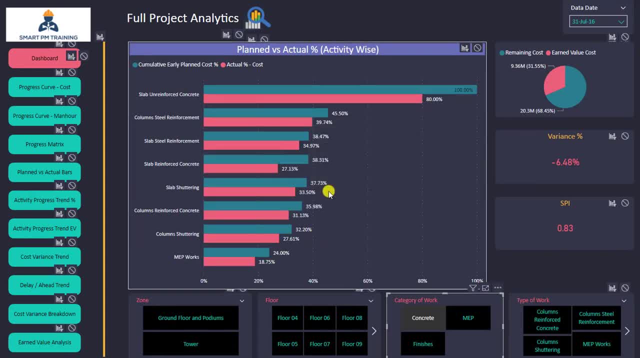 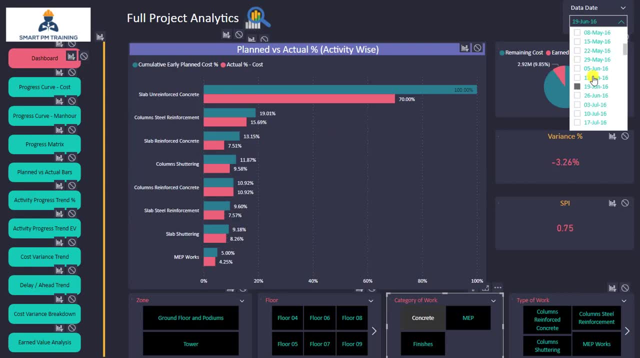 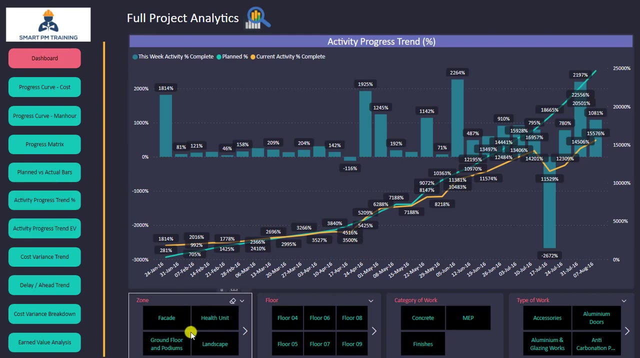 the filters here concrete, for example, and i can see the concrete selection only. also i can change the data date. i will go now to the activity progress percentage trend, which can be very interesting. so first i have to set up my filter. i will choose the ground floor and the podium area. 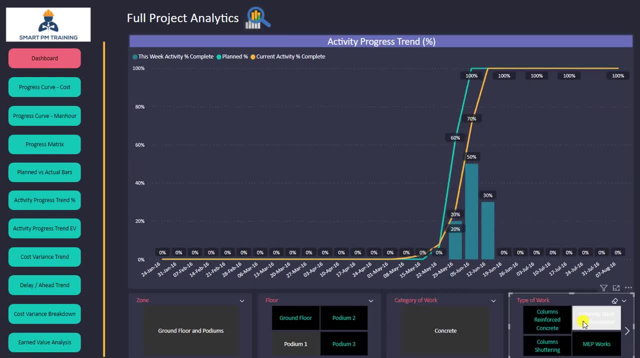 maybe podium one concrete and the column steel reinforcement. it will show me here when the activity has started and what is the progress in each week. so for example, the activity started here, i achieved 20 percent. then the week after i achieved 50 percent of that activity. the last. 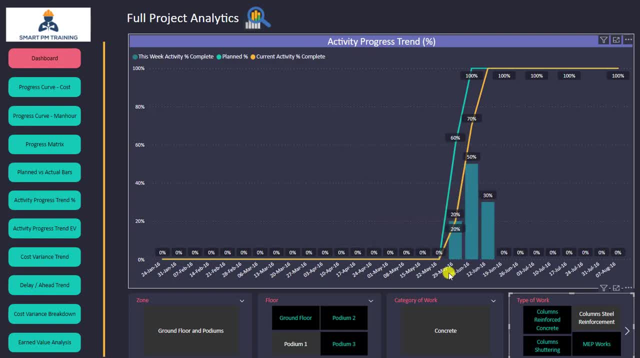 week i finished 30 percent, which means i have completed this activity in three weeks period. i can see also the cumulative at each point. so for example, in the second week i achieved 50, but overall 70 percent of that activity. then i completed the activity a hundred percent in my third week. i can also compare it with the plant. i can see: 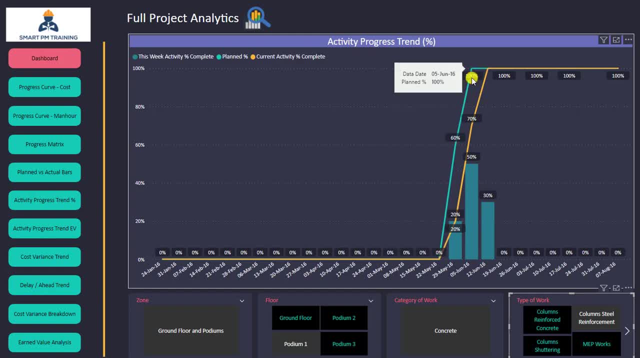 that i started late because the planned line is shown here and at each week what is expected from me to accomplish. so this can be very, very valuable to review, with the trend over particular activity, not only the cumulative status or the overall, but also what's happening in my trend. i will go now to the progress. 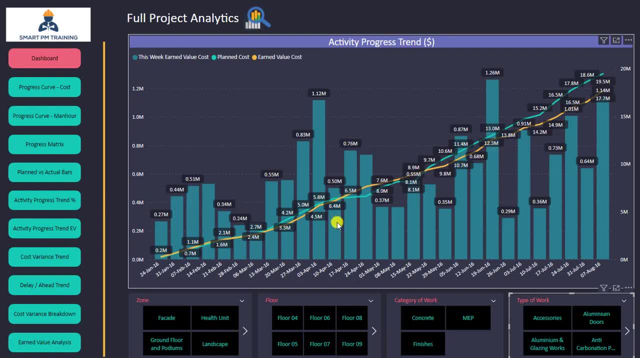 trend based on earned value. so it is similar to the previous visual. however, it's showing me the earned value analysis, not the activity percentage, so right now i can see on weekly basis how much i have achieved. what is the cumulative actual? what is the cumulative plant? but based on the earned value cost. 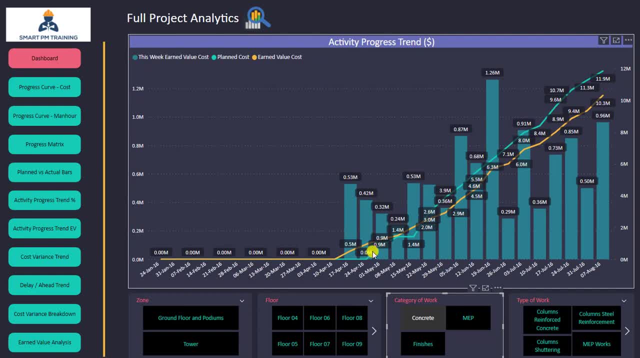 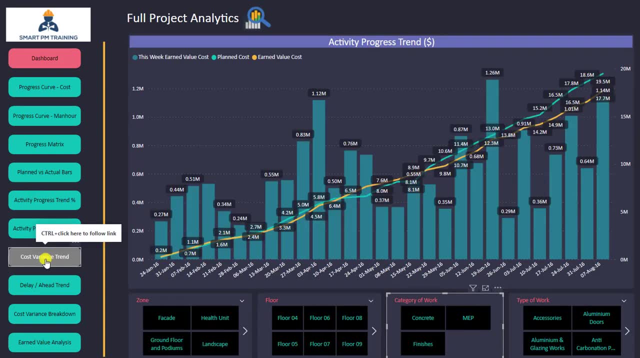 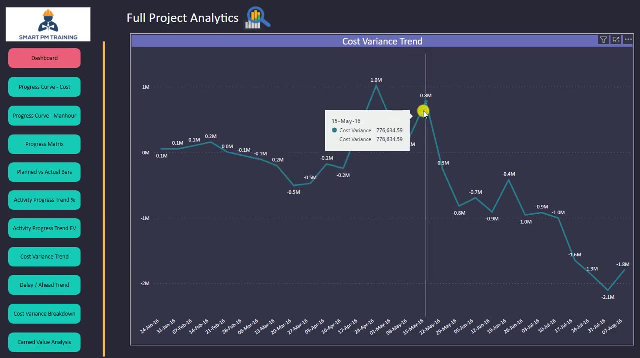 i can also go to concrete, for example, and the chart is automatically updated. i can use the whole ground floor and the podium area. i can do whatever i want. finishes, and this is my cost variance trend. so how much i am falling behind the planned progress? so this is my cost variance itself over time and i was a little bit ahead. 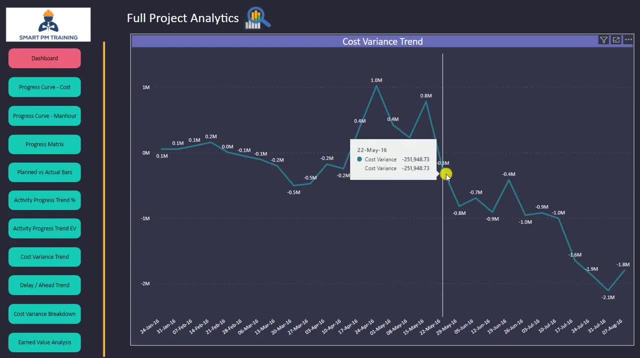 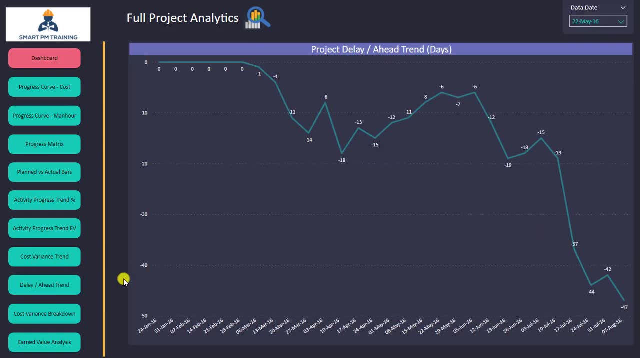 here during this period, then it has been fluctuating with me. then from this point onward, the cost variance is increasing over time. delay and ahead trend. the concept is similar to the previous chart, but this time i'm showing the project delay in amount of days and not cost variance. so i was here on 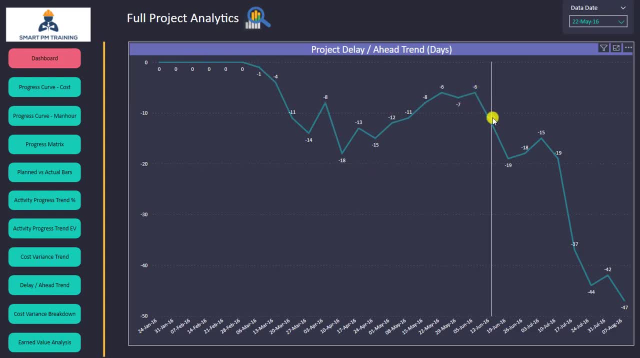 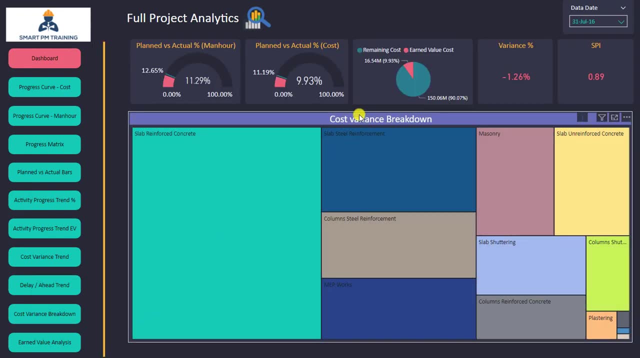 schedule, but it has been fluctuating a little bit. then the delays increase. from this point onward i can go to the cost variance breakdown, because i know right now what is the cost variance for the whole project and i wanna know where the highest cost variance is located in my project. this chart is automatically updated for me. 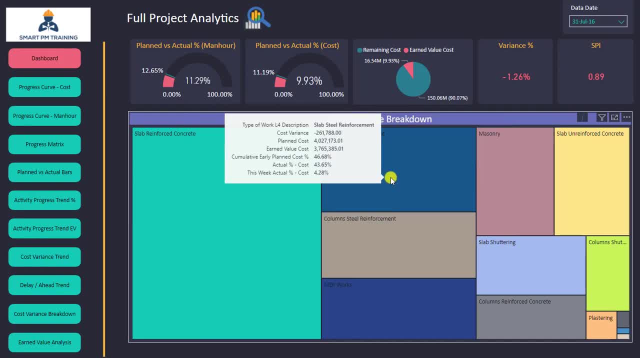 the highest cost variance is located in this area, followed by this area, then this activity, then this activity, and so on. i can also hover on any activity and i will see additional information, such as planned cost, earned value, cost, planned percentage, actual percentage and what is the actual percentage achieved over the past week only. 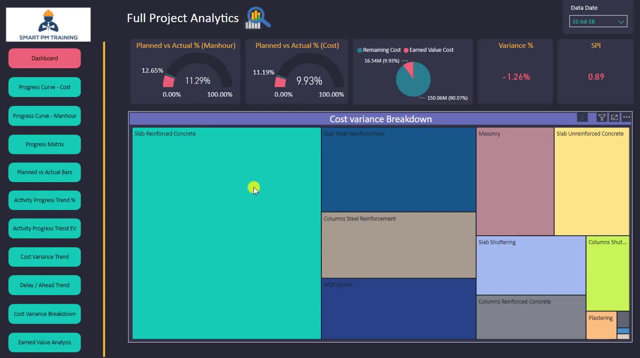 in this case, i want to know if i am getting closer to the recovery or not, and if i select any activity, the indicators are also updated for me, i can see now this activity alone accounts for the highlighted area and the earned value cost from the whole project. 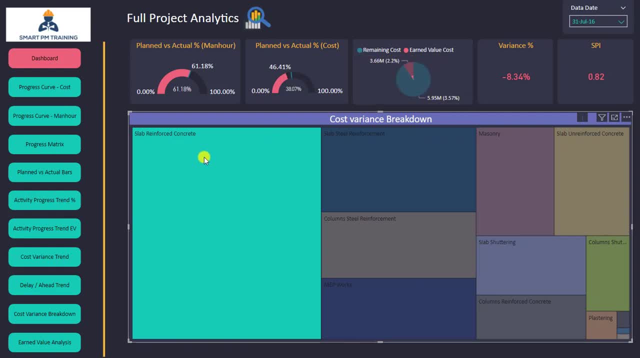 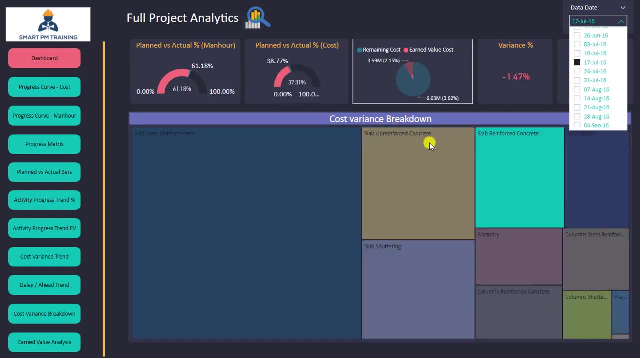 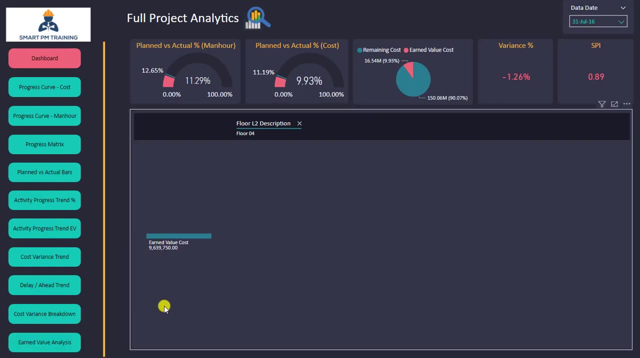 and the figures here are updated as well- for the slab reinforced concrete only and, as we have seen before, i can always go back and check the progress status on any data date. so this is very powerful and here i have the earned value cost from this button. i can click the plus sign here and i can see: